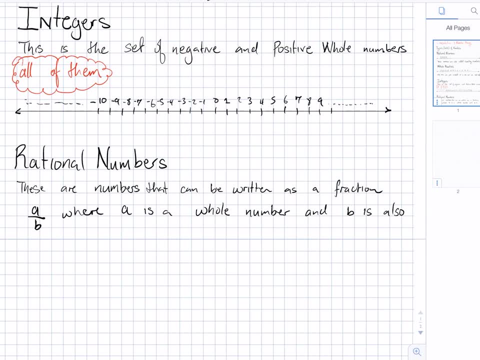 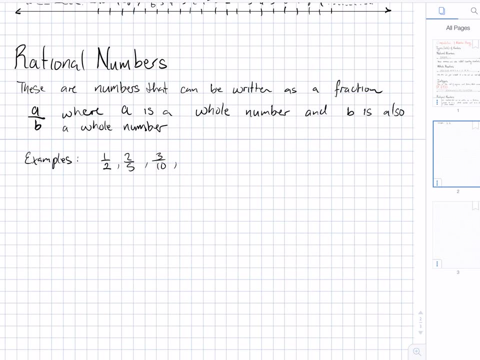 a whole number and b is also a whole number. Examples: 1 divided by 2,, 2 divided by 5,, 3 divided by 10,, 10 divided by 3,, 7 divided by 6,, 4 divided by 2,, 8 divided by 9, and so on. 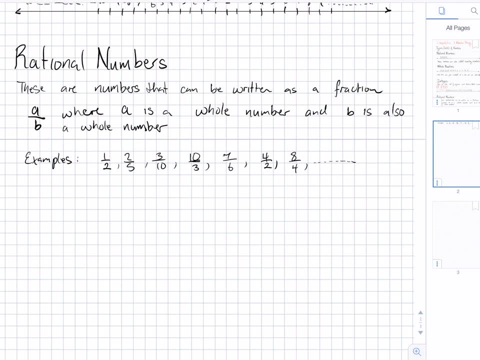 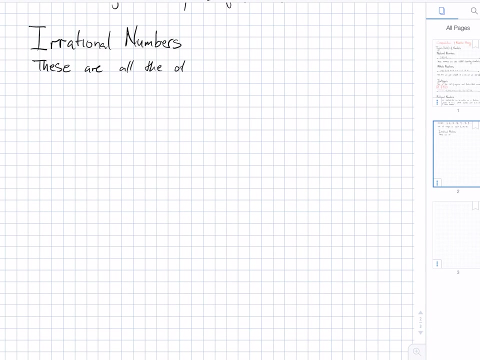 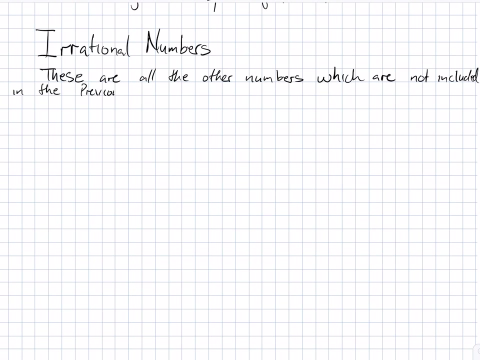 Note: all integers are a part of this set, So the next set of numbers that we move on to are the irrational numbers. Irrational numbers: these are all the other numbers which are not included in the previous sets, So to remember them, I always say that they are special, non-recurring decimals right Special. 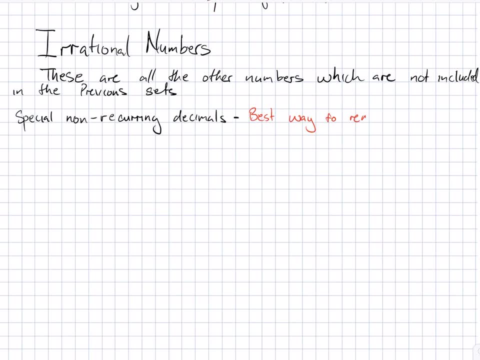 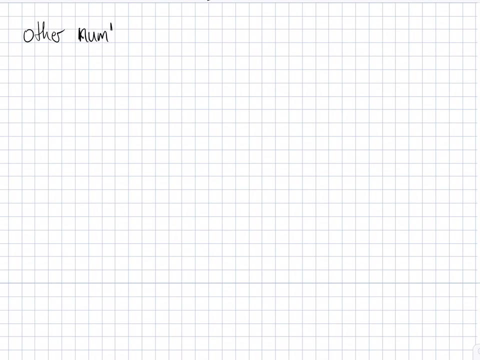 non-recurring decimals. Example: the number e, the number pi, square root of 3, the square root of 5, or even the square root of 2, the list goes on. Other number sets which we have not included in our previous sets are the even numbers. 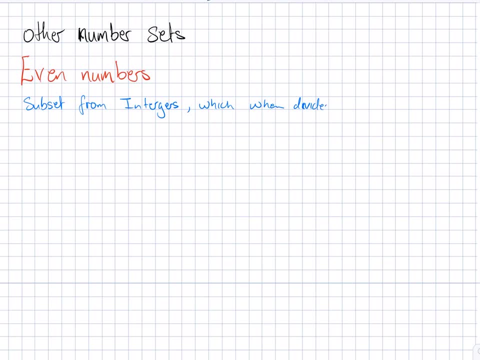 right, And the even numbers is actually a subset from the set of integers which, when divided by 2, the remainder is 0.. Example: negative 6, negative 4, negative 2, 0, and it's important to know that 0 is an even number. 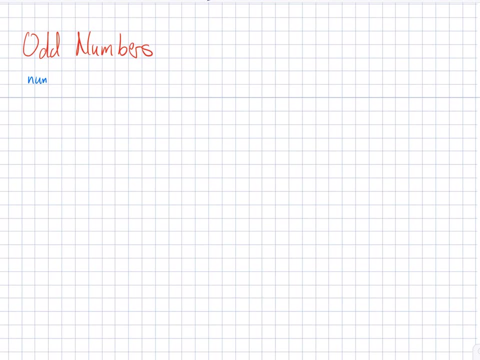 Next we move on to the set of numbers, of odd numbers, and I'll define the set of odd numbers to be the set of numbers that are not even and they are also in the set of integers. So those set of integers which are not even are said to be odd and we can represent this on a 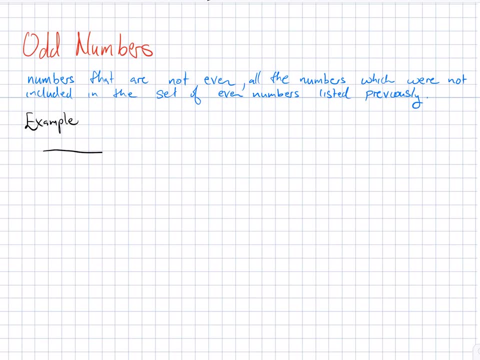 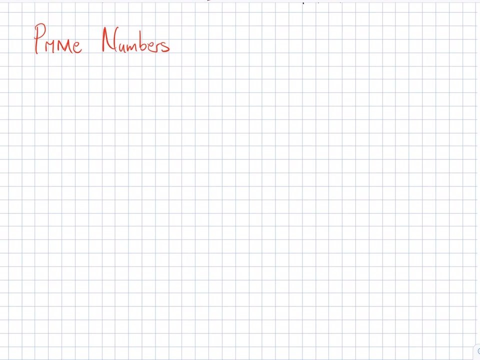 number line by looking at the numbers negative 7, negative 5, negative 3, negative 1, 1, 3, 5, 7, 9 onwards. Another unique set of numbers that also comes up a lot in mathematics are the set of prime numbers, and these are numbers: 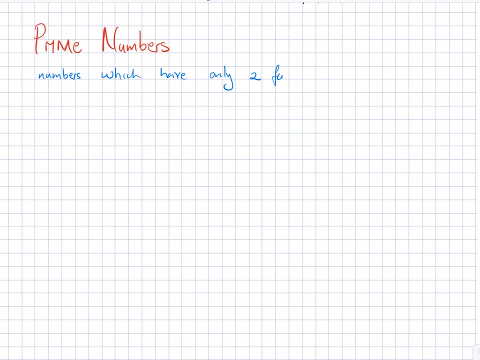 which have only two factors, one and itself: Examples 2,, 3,, 5,, 7,, 11,, 13,, 17,, 19,, 23,, 29,, 31,, 37, just to name a few. Note that one is not a prime number, right and. 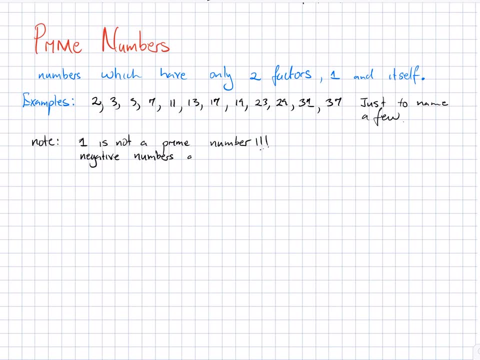 negative numbers are not prime either. The next set of numbers which will be looking at are composite numbers, and these numbers are whole numbers which are greater than 2 but are not prime. Examples: 4, 6,, 9,, 8,, 18,, 15,, 22 and so on. 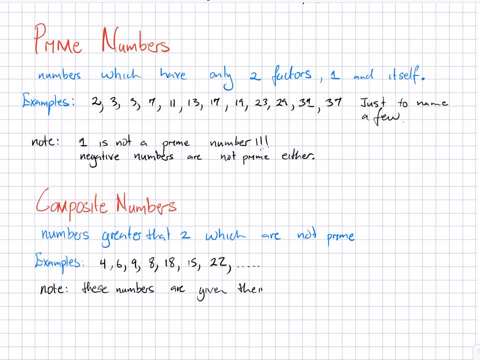 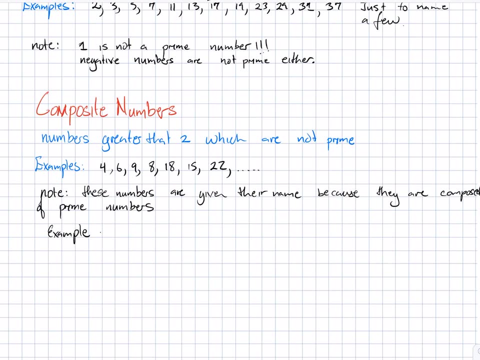 Note that these numbers are given their name composite numbers because they are composed of prime numbers. Example: the number 4. if we should factorize the number 4, we can write it as 2 times 2.. Note that both of these factors are prime. I can take the number 8 and. 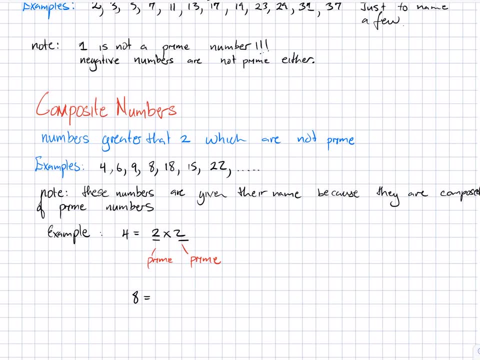 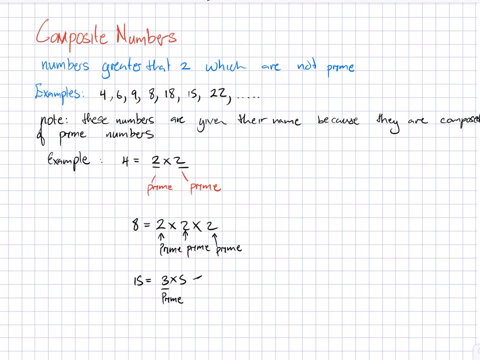 factorize the number 8 as 2 times 2 times 2 and note that all the factors are prime. The number 15 is composed of 3 times 5, which are both prime numbers. so we see that all composite numbers can be factorized into prime factors. That's a. 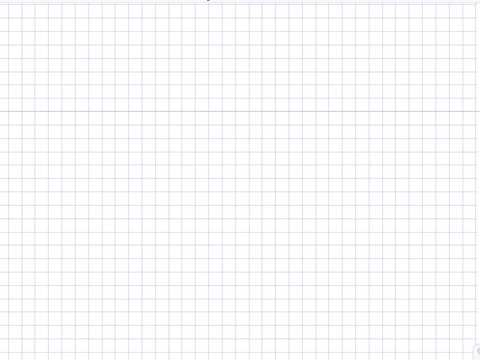 very important note. Next, we move on to the order of operations, and across the globe the order of operations is referred to as different names. Some people call it BOMDAS and some people call it PEMDAS, Where BOMDAS stands for Bracket of Multiplication, Division, Addition and 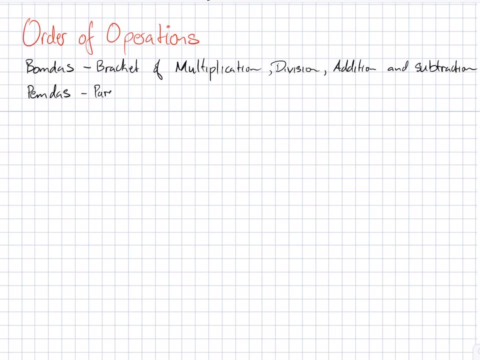 Subtraction, while PEMDAS stands for Parental Expressions, Multiplication Division, Addition and Subtraction. Now, to demonstrate the order of operations and how to use it, we'll be looking at the evaluation of expressions involving integers. Alright, so let's take some basic examples. 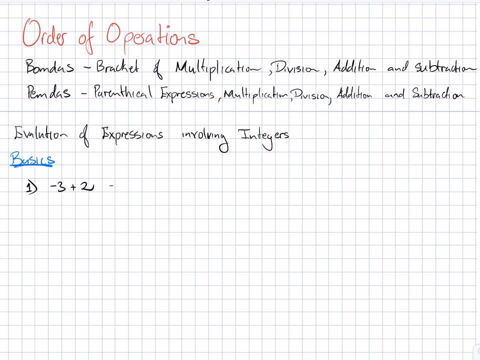 Example number 1, negative 3 plus 2 is equal to negative 1, and it's important to note that when the signs are different, we subtract and keep the sign of the bigger number. So here we're working with negative 3 and a positive 2, so we're going to subtract. 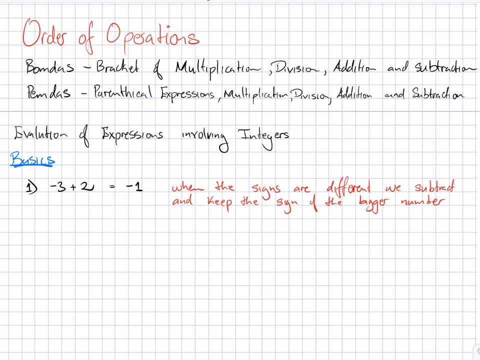 that 3 minus 2 is actually 1 and the sign of the bigger number is negative, so the result is a negative 1.. Example number 2, we have negative 5 minus 7, which is equal to negative 12. We want to note that when the signs are the same, we add and keep the sign. so here, if you, 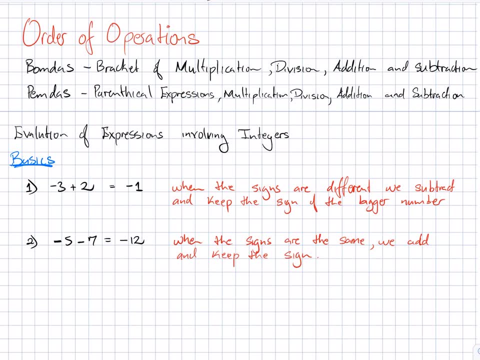 add 5 and 7, the result is 12 and if we're keeping the sign, it's a negative 12.. Example number 3, we look at the expression negative 2 plus 4, which is equal to 2, since 4 is the bigger number. when we subtract 2 from 4, we end up with 2 and we keep the sign. 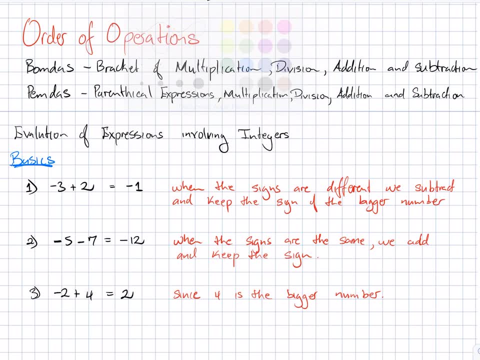 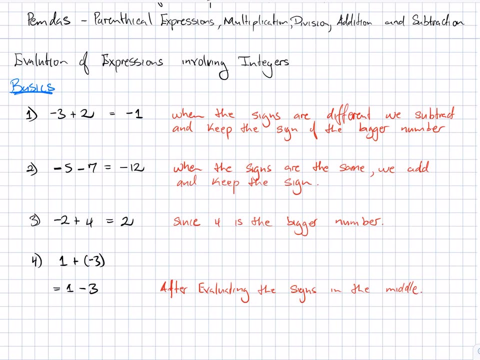 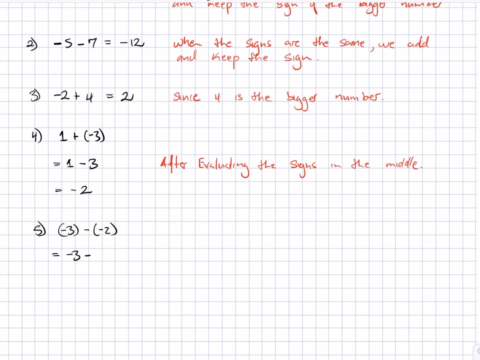 of 4, which is a positive 2.. Example number 4, we have 1 plus a negative 3, which is equal to 1, minus 3, which is equal to negative 2, after evaluating the signs in the middle. Now we look at example number 5, we have negative 3 minus negative 2.. Here the signs in the middle: 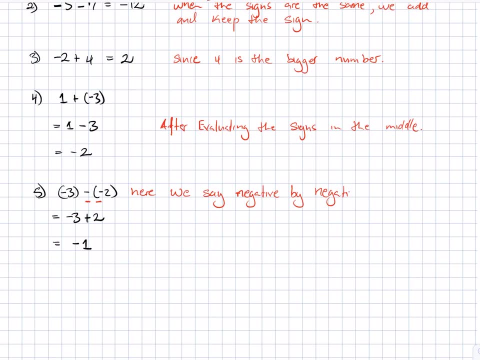 are both negative, so we can change that to a positive, thus becoming negative 3 plus 2, which is equal to negative 1, which simplified down to our first example, Example number 6, we have 2 plus negative 7, which is equal to negative 7.. So if we subtract that, the 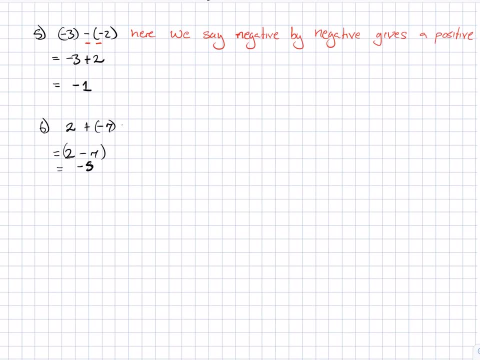 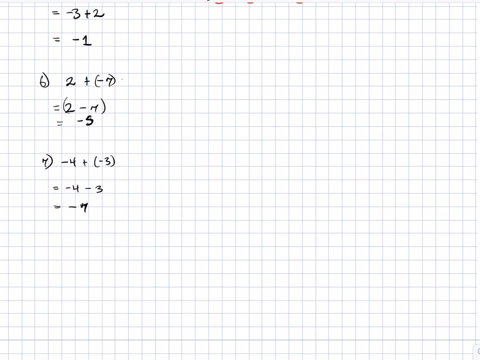 which is equal to 2 minus 7,, which is equal to negative 5.. Example number 7, negative 4 plus negative 3 is equal to negative. 4 minus 3,, which is equal to minus 7.. Example number 8, minus 5 plus 7 plus negative 3,. 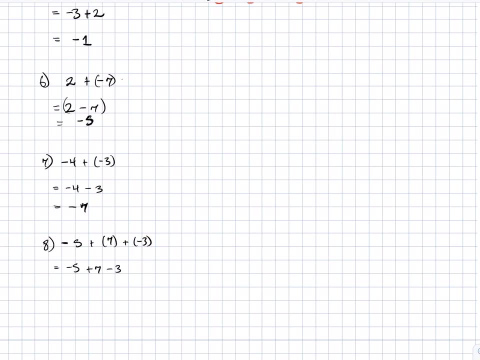 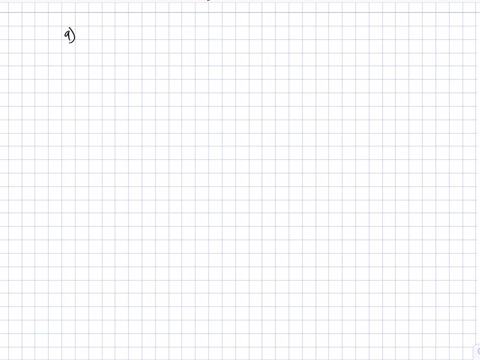 which is equal to negative 5 plus 7 minus 3,, which is equal to negative 5 plus 4,, which equates down to negative 1.. Example number 9, here we're looking at multiplication. We have negative 1 times 3,, which is equal to negative 3.. 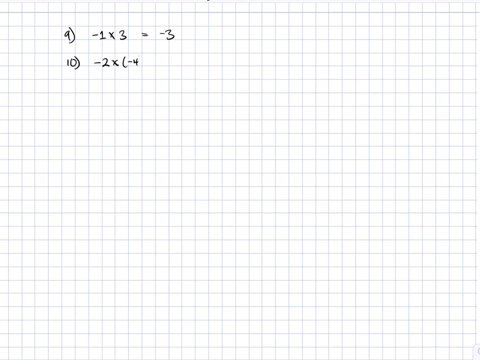 Example number 10, negative 2 times negative 4 gives us a positive 8.. Example number 11, 8 divided by negative 4, right. We want to note that here, positive divided by a negative gives a negative. So when we take 8 and divide it by negative 4, the answer is negative 2.. 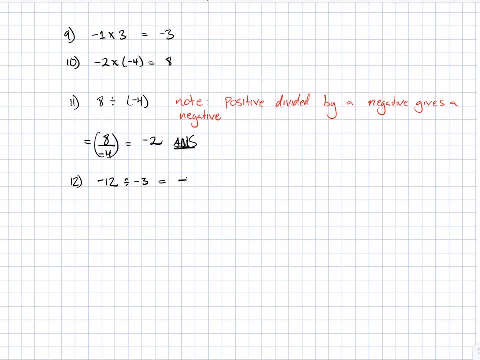 Example number 12 is negative 12 divided by negative 3, right. And when a negative is divided by a negative, the answer is positive. So this negative 12 divided by negative 3 is going to give us a positive 4.. 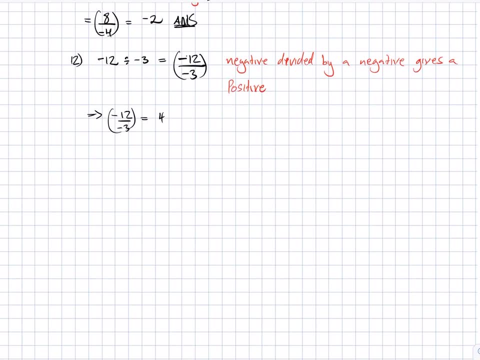 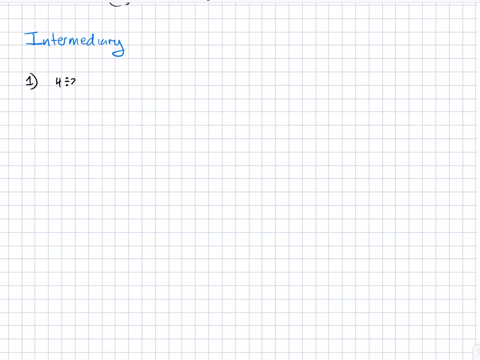 Next we move on to the intermediary form, Where we have brackets involved in the expression. Take example number 1, 4 divided by 2 in bracket, multiplied by 2 minus 3 in bracket. The first thing we want to do is evaluate the expressions inside the bracket. 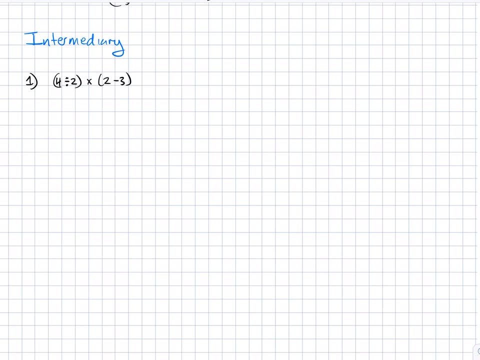 or the expressions inside the parentheses. So this will give us 2 for the first expression, times negative, 1 for the second expression and 2 times negative. 1 is negative, 2.. Now moving on, Moving right along to example number 2,. 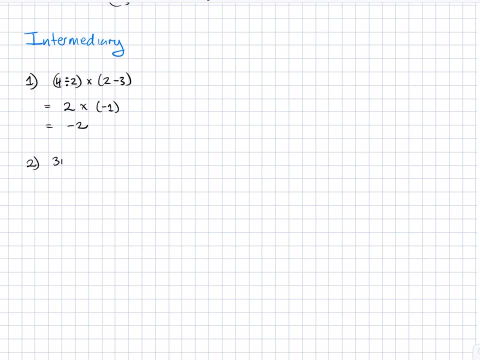 we have 34 minus 17 in bracket, minus 3 times 5 in bracket. We have to evaluate the expressions in the bracket first. So here, 34 minus 17 is equal to 17, and 3 times 5 is equal to 15, thus giving us 17 minus 15,. 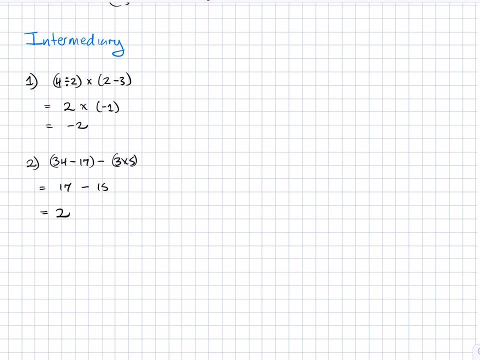 which leaves us with our final answer as 2.. Example number 3 gives us 32 divided by 2 times 4 minus 2 plus 3, in bracket. Evaluating the expression in the bracket first, we realize that 2 plus 3 is 5.. 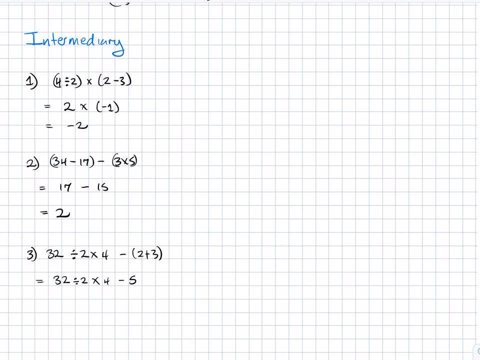 Thus we have 34 divided by 2 times 4 minus 5, and we have to evaluate 2 times 4 first because of order of operations. Multiplication is evaluated before division. This gives us 32 divided by 8 minus 5,. 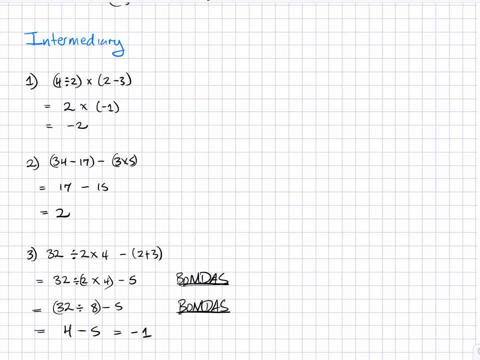 which then gives us 4 minus 5,, which is equal to negative 1.. So we have 32 divided by 2 times 4 minus 5, which gives us 4 minus 5,, which is equal to negative 1.. 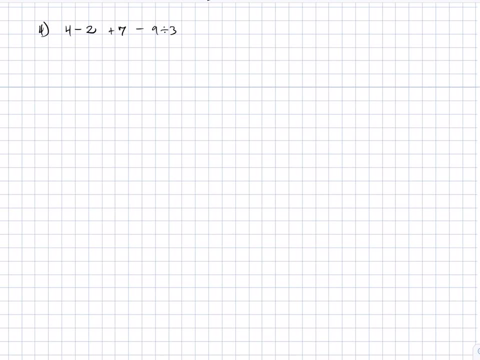 Example number 4, we have 4 minus 2 plus 7 minus 9 divided by 3.. Based on the order of operations, we have to evaluate the 9 divided by 3.. That gives us a 3.. So our next line reads: 4 minus 2 plus 7 minus 3.. 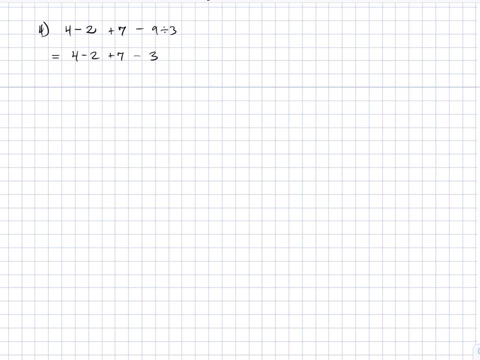 And if we are performing addition first we have to take our 7 and our negative 2, which gives us 7 minus 2, or negative 2 plus 7,, which gives us 7 minus 2, or negative 2 plus 7,. 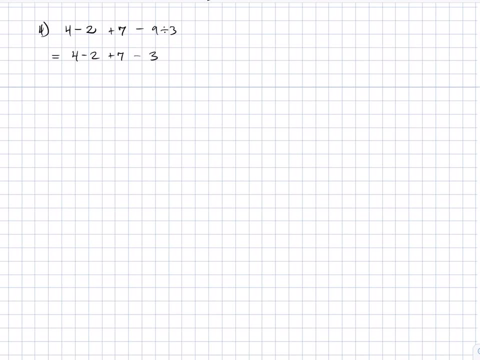 which gives us 7 minus 2,, or negative 2 plus 7,, which works out to 5.. So our next line reads: 4 plus 5 minus 3,, which is equal to 9 minus 3,, which is equivalent to 6.. 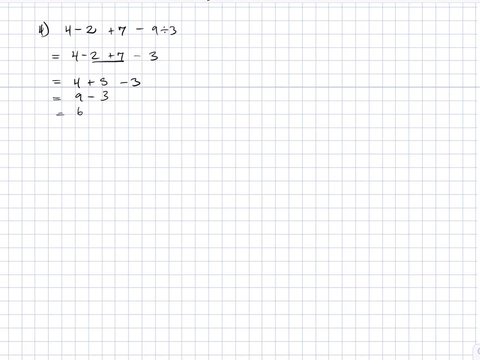 There are other variations of this solution, but the final answer should come out to 6.. Example number 5, we have 3 divided by 3 in bracket, plus 4 times 2 in bracket, minus 6 divided by 2 in bracket. 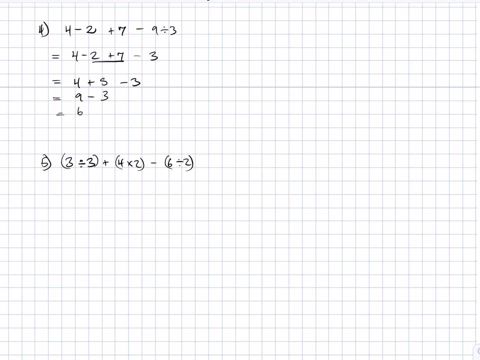 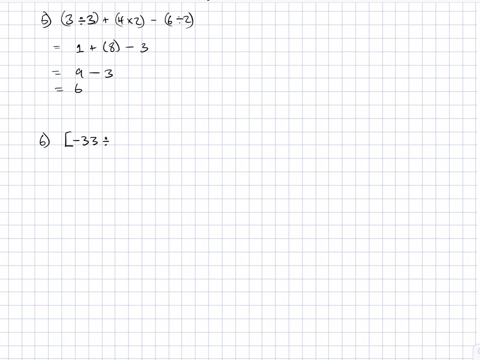 Based on the order of operations, we have to evaluate the expressions in the bracket First, which gives us 1 plus 8 minus 3, which is equivalent to 9 minus 3, which is equal to 6.. Example number 6, we have in bracket negative 33, divided by negative 11. 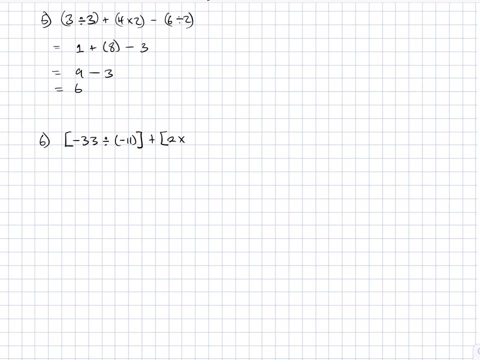 plus 2 times negative, 3 in bracket, plus negative, 2 times negative, 3 in bracket, which gives us 3 for the first expression plus negative, 6 for the second expression, plus positive 6. For the last expression, if I should evaluate this, 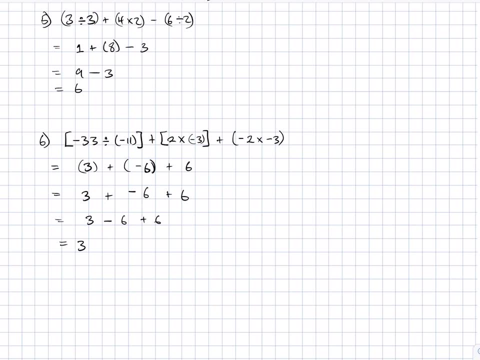 we would get 3 plus negative, 6 plus 6, which is equal to 3 minus 6 plus 6,, which is equivalent to 3.. Example number 7, we have 9, take away 12 divided by 3 times 2.. 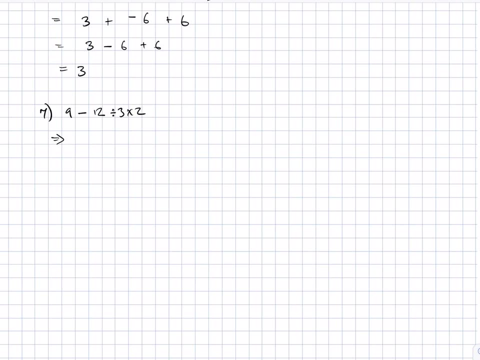 Following the order of operations, we have to do multiplication first, so this gives us 9 minus 12 divided by 6.. And then our second operation should be division. so we have to take our 12 divided by 6, which gives us 2, which means our next line reads: 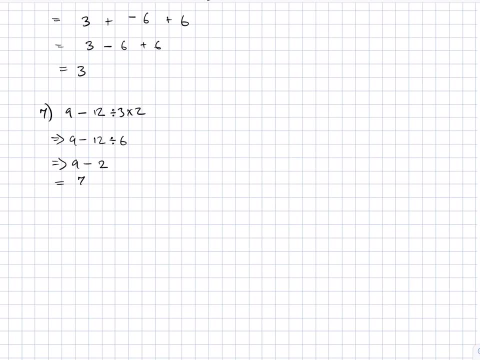 9 minus 2, which is equal to 7.. Example number 8, which is our final example before we move into number theory, part 2,. we have 8 plus 14 divided by 7, plus negative 2 times 7 in bracket.